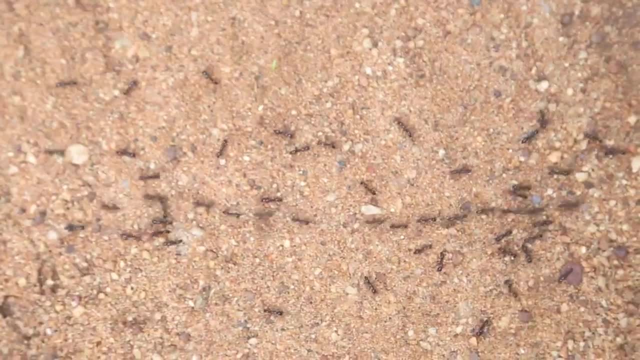 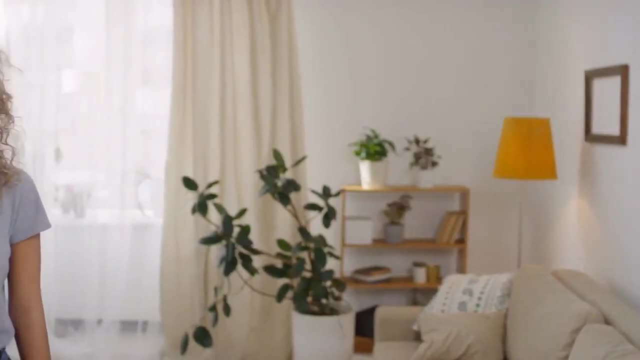 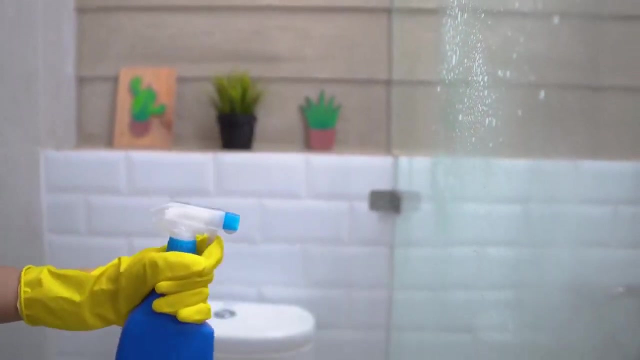 Glass cleaner and liquid detergent. Ants leave a scented pheromone trail behind when they walk, which acts as a map. This method can remove the scent and deter the ants from re-entering your home. Here is how to do it: Mix glass cleaning spray with liquid detergent. dish soap into a 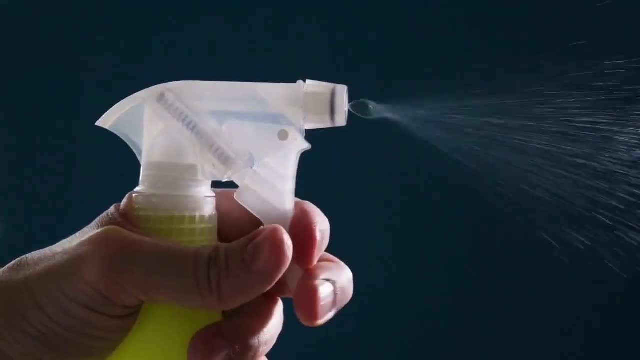 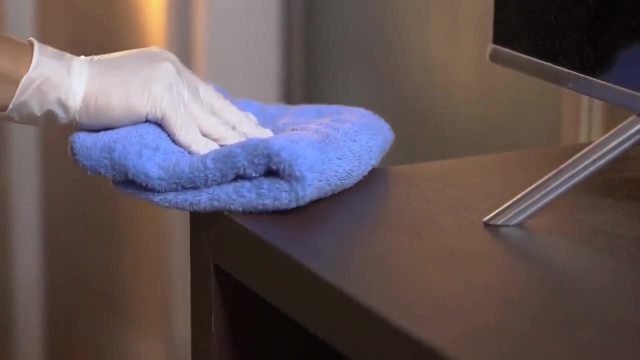 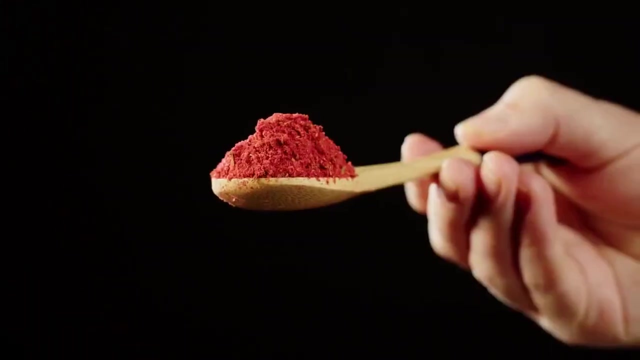 clean spray bottle. Spray the mixture on areas where ants seem to enter. After spraying, wipe down the area, leaving a light residue. Repeat the above steps as often as needed. Ground black or red pepper. Black or red pepper is a natural ant deterrent as the insects 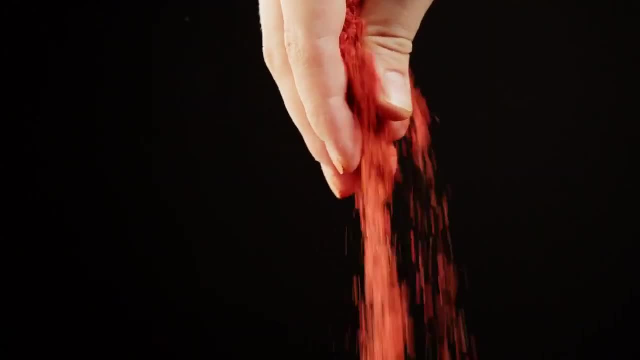 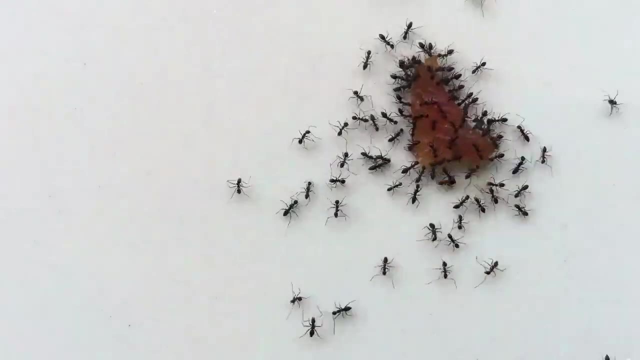 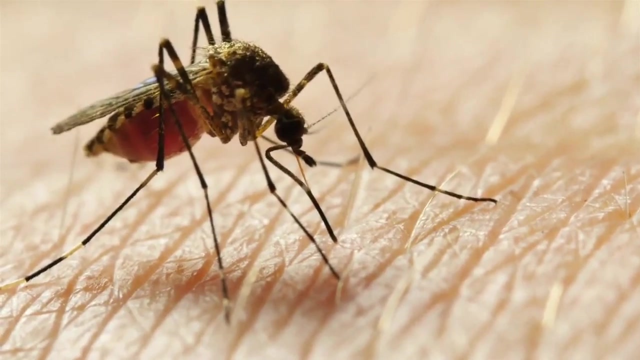 appear to find the smell irritating. To use this method, sprinkle pepper around baseboards and behind appliances. Anecdotal evidence suggests that this is a safe way to help keep ants at bay. Peppermint- Peppermint is a natural insect repellent that may effectively deter ants and 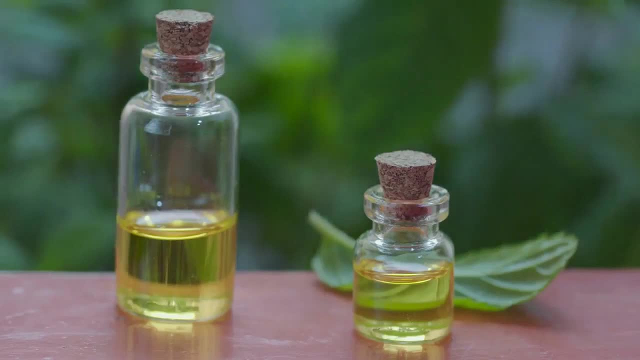 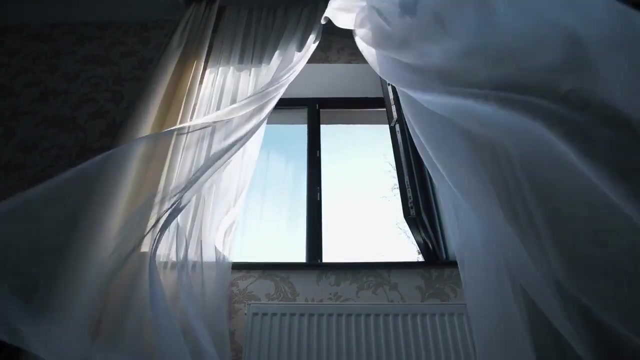 other bugs, such as mosquitoes, To use peppermint essential oil as an ant deterrent. complete the following steps. Mix 10 to 20 drops peppermint essential oil with 2 cups water in a clean plastic spray bottle. Spray the mixture around the baseboards and windows of your home. 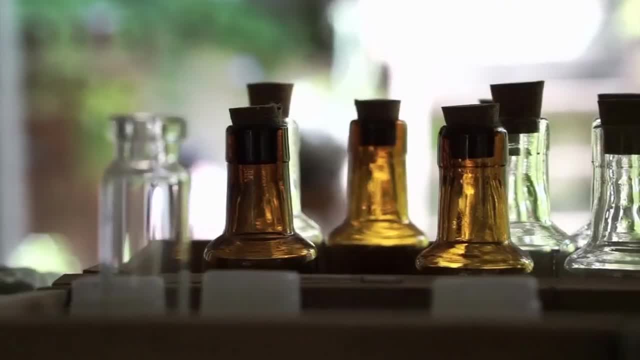 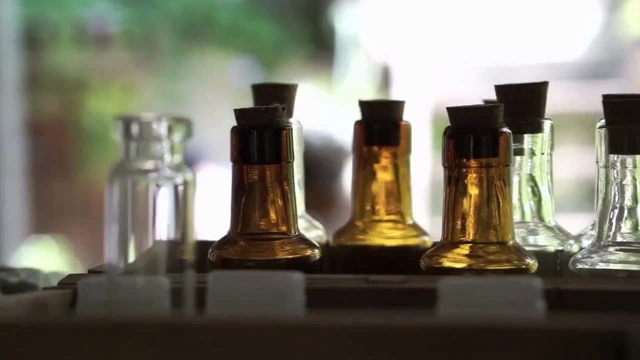 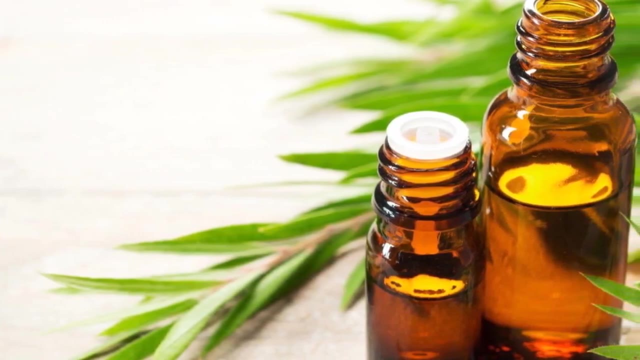 Allow the mixture to dry and repeat as needed. Like most essential oils, keep peppermint oil out of reach of pets, especially cats, which can become very ill if exposed Tea tree oil. Like peppermint oil, tea tree oil can be an effective ant deterrent To use this method. 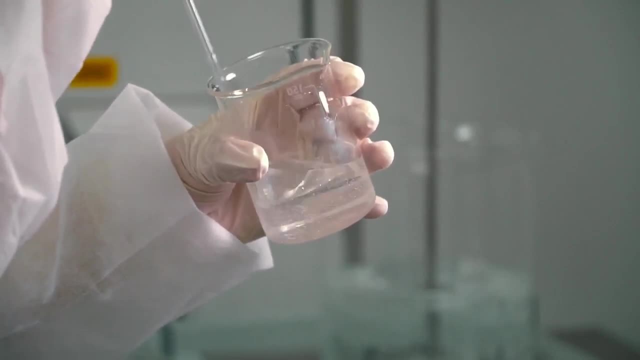 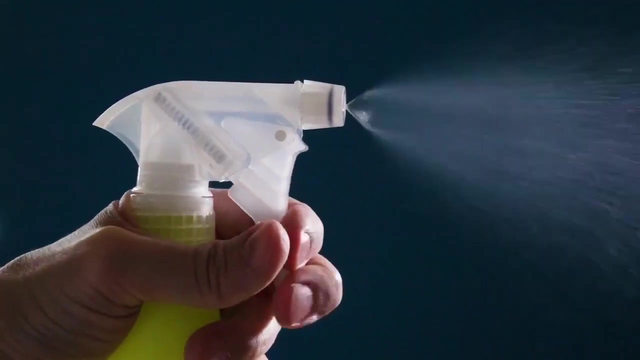 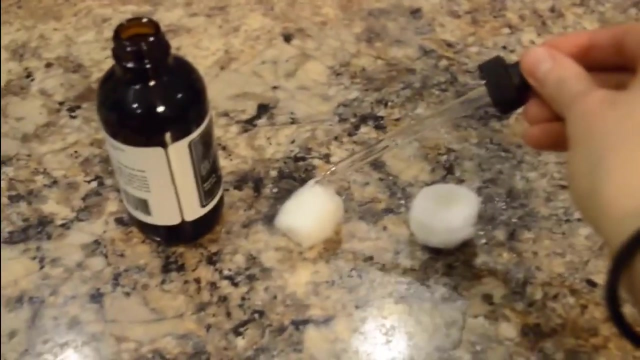 complete the following steps. Mix 5 to 10 drops tea tree essential oil with 2 cups water in a clean plastic spray bottle. Spray the mixture around the house where you typically see ants. Alternatively, you can prepare the tea tree to use as a lamp or for light space. 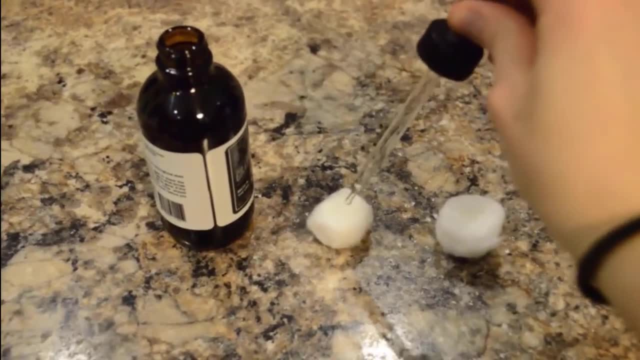 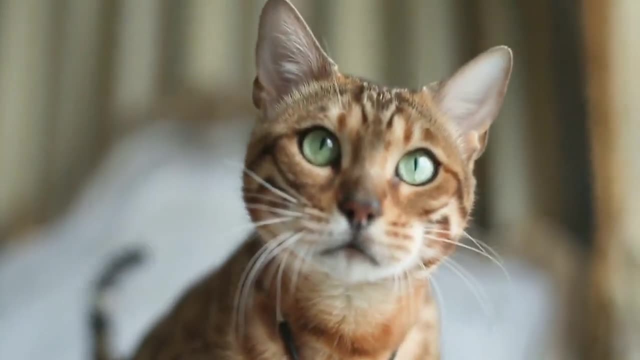 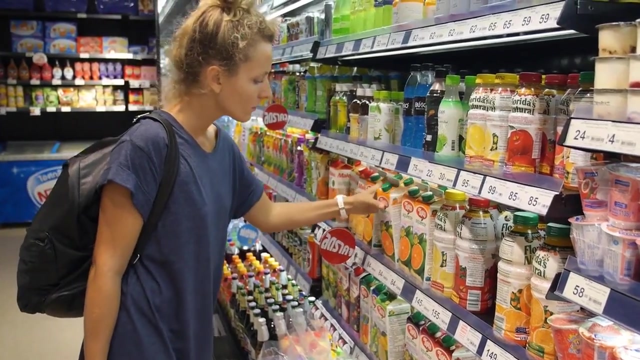 Use a kitchen towel to help clean the tea tree. Do the following steps as the following: Put tea tree oil on the floor and place the bowl with the mixture around your home. Like most essential oils, keep tea tree oil out of reach of pets. 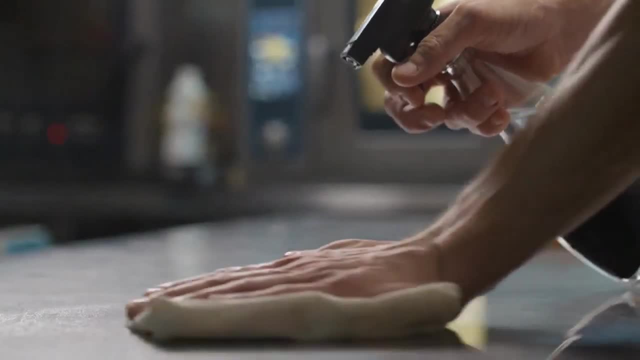 White vinegar. White vinegar, available at all grocery stores, is a cheap and effective way to kill and repel ants. It is also a natural cleaning agent. Try using a white vinegar for drinking water, or instead use a non-phosphorus or citric acid water or vitamin E. 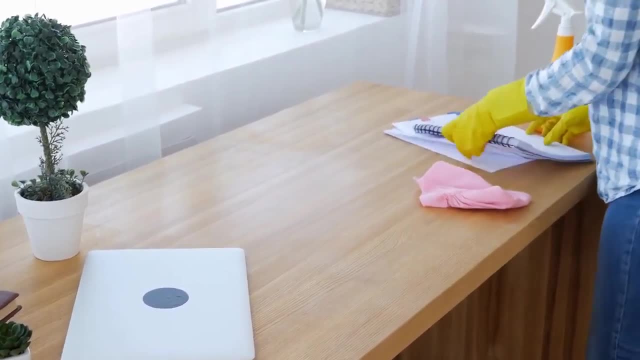 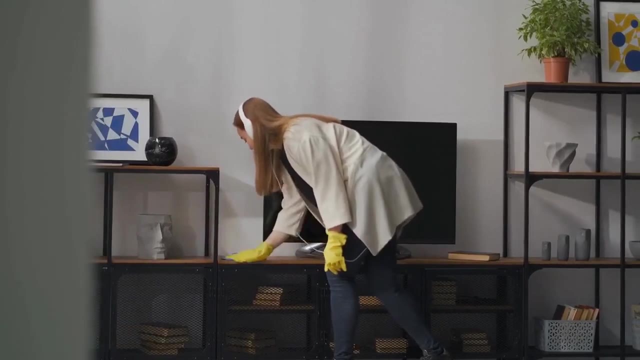 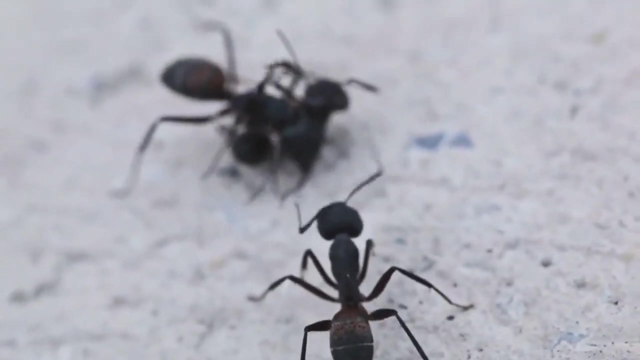 one-to-one vinegar-slash-water mixture to clean hard surfaces, including floors and countertops, wherever ants are likely to travel. If you see ants, spray the mixture on them or wipe them up with a paper towel. Ants can smell the vinegar after it dries, but the scent doesn't remain. 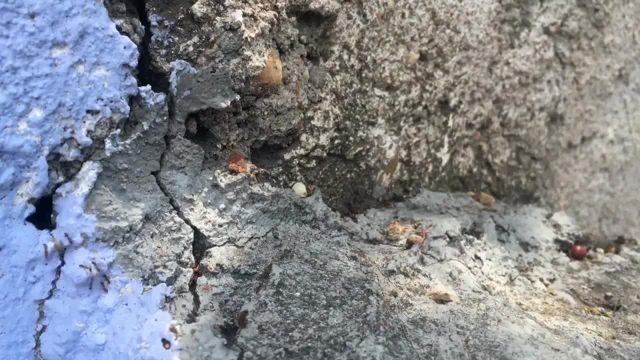 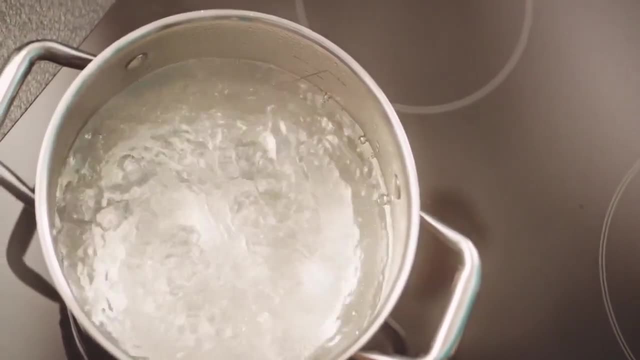 long for most people- Boiling water. If you notice ant holes near your home, pour boiling water into them, This method will effectively and immediately kill. many of the ants inside Ant hills may appear small, but the ant colonies underneath them are vast. The boiling water won't be enough to kill. 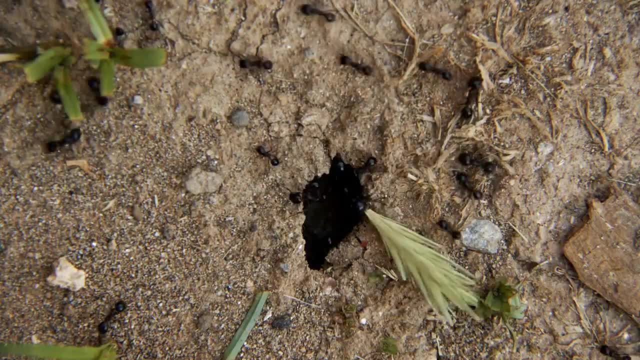 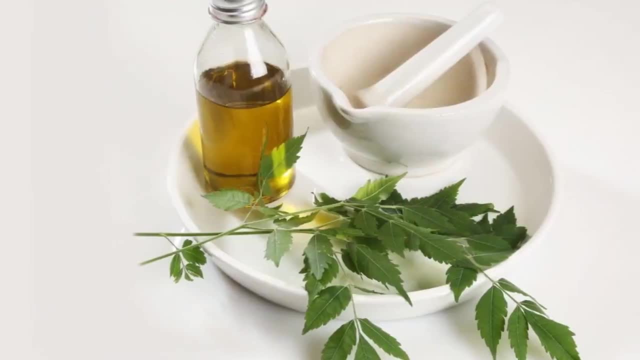 off the entire colony. For this reason, make sure to treat every ant hole you see within your home's proximity. Neem oil: Neem oil is a naturally occurring insecticide extracted from the neem tree native to India. Gardeners recommend. 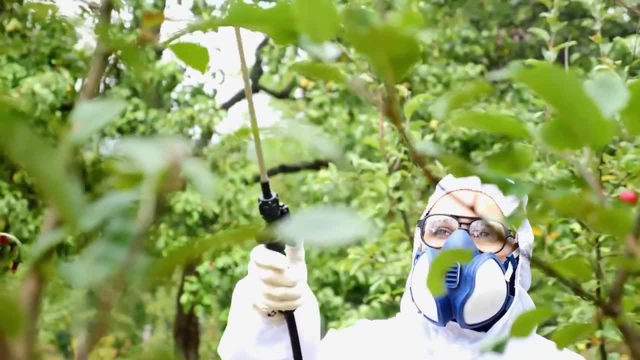 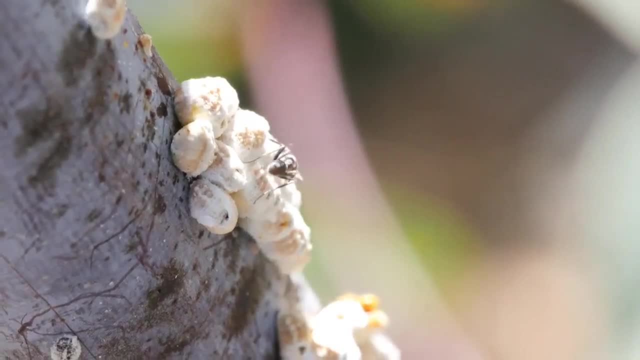 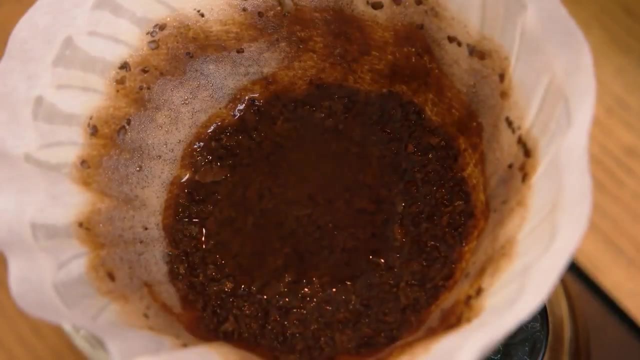 using neem oil around plants, especially where you see aphids or ants. Ants, farm aphids- small sap-sucking insects, so poisoning the aphids with neem oil can take care of both types of pests. Coffee grounds- Brewed coffee grounds- have been found to detract ants. Try sprinkling the freshly. 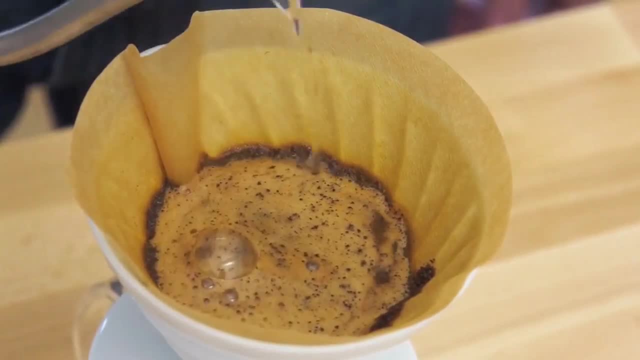 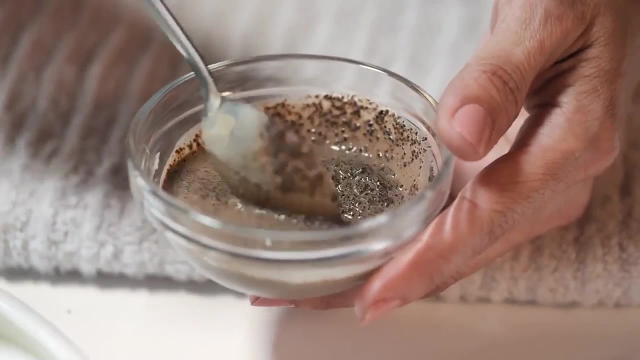 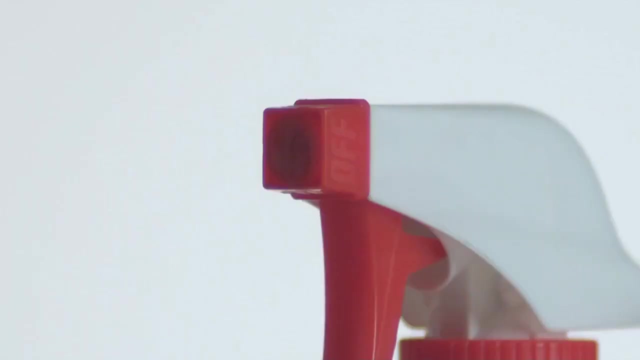 brewed coffee grounds on disposable surfaces and leaving them in areas where ants congregate, such as pet bowls. You can also place the grounds on window sills. The grounds may lose their potency once they're dry, so make sure to change often Lemons: You can spray or wipe lemon juice to detract ants by removing pheromone trails. 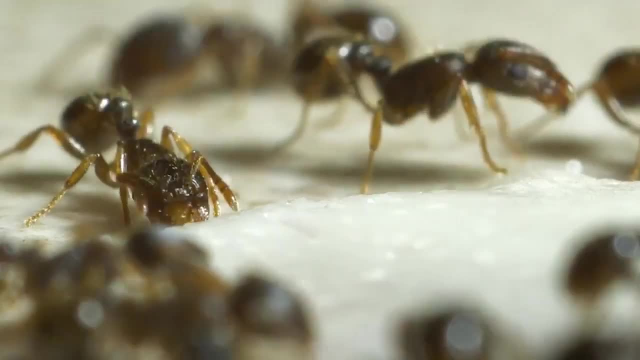 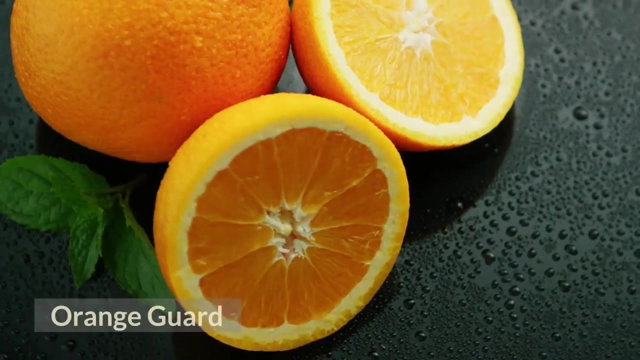 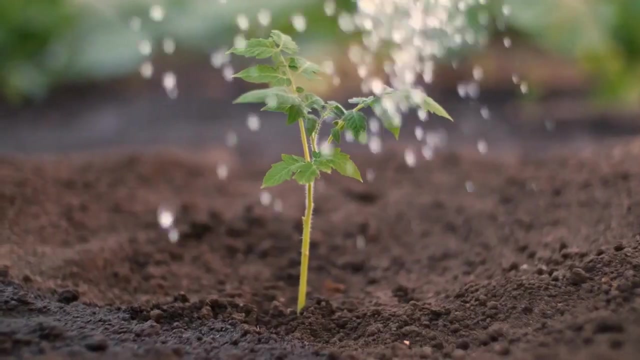 and masking the scent of food. In addition, putting lemon rinds in your cupboard may also detract ants from taking up residence in your kitchen. Orange guard: You can actually purchase an orange peel spray or make your own DIY citrus spray. Citrus peels contain a natural extract, D-limonene, which is not harmful to the 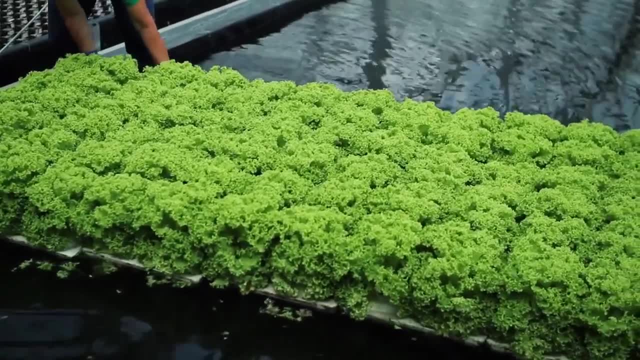 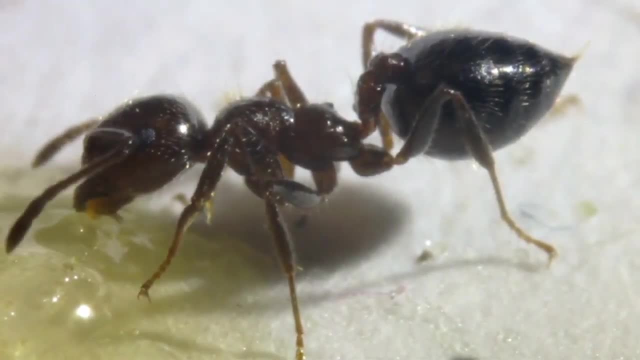 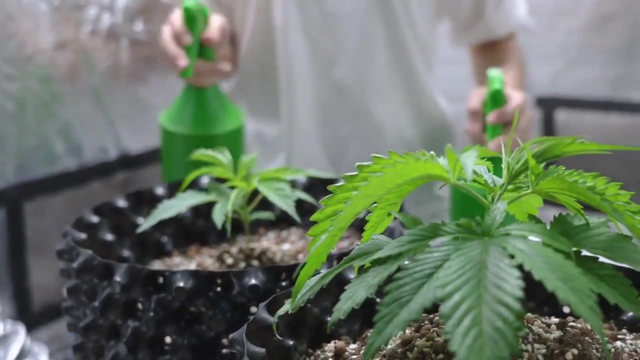 environment or the soil. This is a food-grade product, so safe for vegetable gardens. This immediately strips away the waxed coating on ants, causing them to suffocate. Dawn dish soap spray. Mix dawn soap and water and put into a spray bottle.